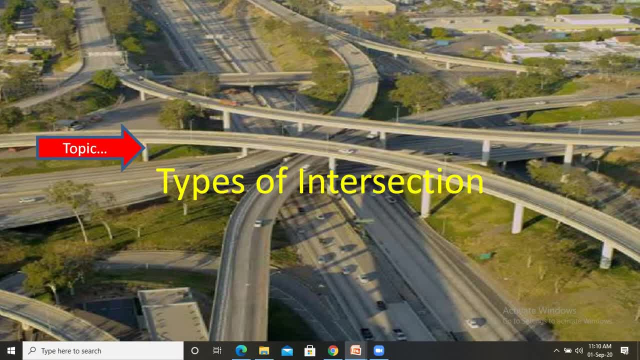 So in remaining case, apart from these two cases, we cannot avoid the traffic problem or intersection problem. So that's why we need to build different kinds of construction, is there? Such problems are avoided by providing grade separate intersection and controlled access. So then only we can overcome these intersection problem guys. 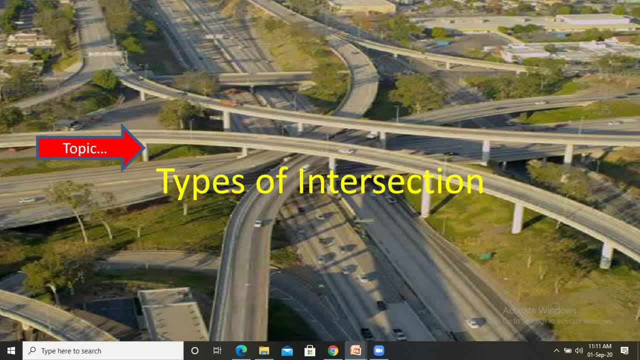 So the efficiency, safety, speed, cost of operations and capacity of road road system very much depends on intersection design. Obviously, these are the very necessary points And pedestrian movements at intersection processes are increased, provide hazards and delays. So these all those things we need to require, guys here. 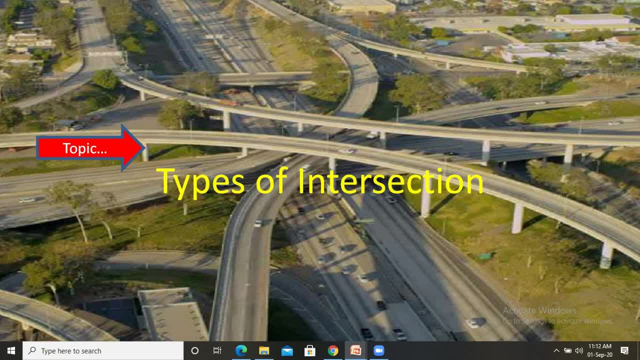 So safety we need to require. speed is good and we need to require efficiency, we need to require and cost of operation. These all those things we can provide in a good manner That only we can do. Avoid the is kind of the problems at particular position. 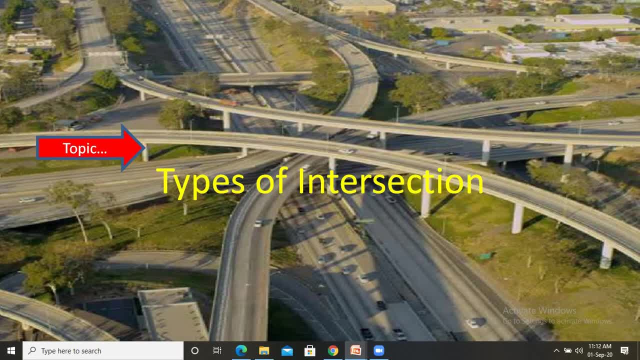 So this is the information, guys, regarding intersection. So we can, we should avoid. our motto is: we should avoid the traffic problem at the intersection zone, means at junction zones. we need to avoid. So basically, in our construction, So generally our Indian construction is 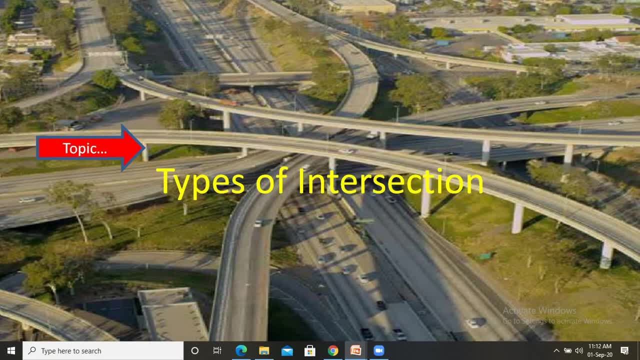 So basically in our construction, So generally our Indian construction is, So basically in our construction There are 90% maximum, 90% integrated intersection only. so every road meeting at a particular junction, At that point only we have separate the travelling or what ever it be. 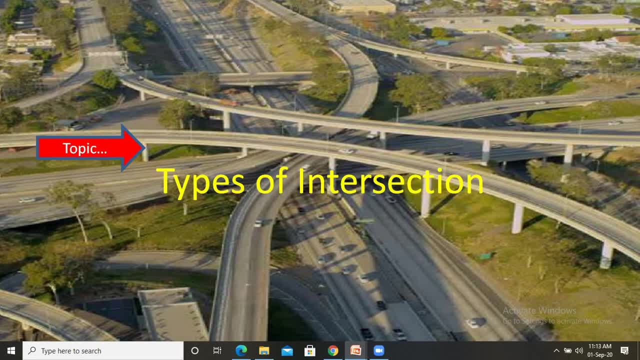 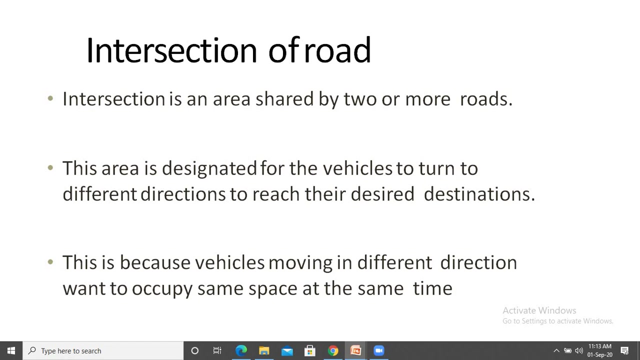 So if we are providing the great separate intersection, we can automitically overcome the problems at intersection zone. So we will discuss some of the things from this intersection topic. So, guys here, types of intersection we will discuss here. so intersection is an area shaded by two or more. 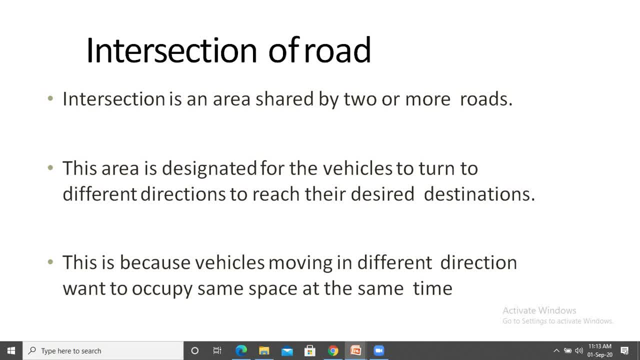 roads. so obviously that is correct- two or more roads shared by at a particular location or whatever it may be. so that is we can say intersection of road. this area is designated for the vehicles to turn to different direction to reach their desired destination. yes, so for example, we are traveling from a to b. at b point there is a junction, is there? so we need to move. 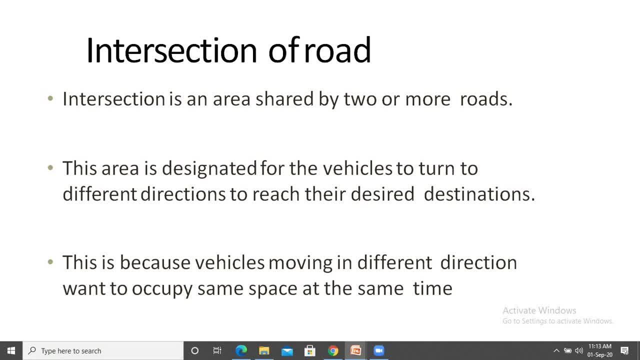 from b to d direction. so we cannot move directly from a to d, so we should come at a junction point. at that time we need to turn and we need to move our destiny point. so that's why we are using the intersection and this is because vehicle 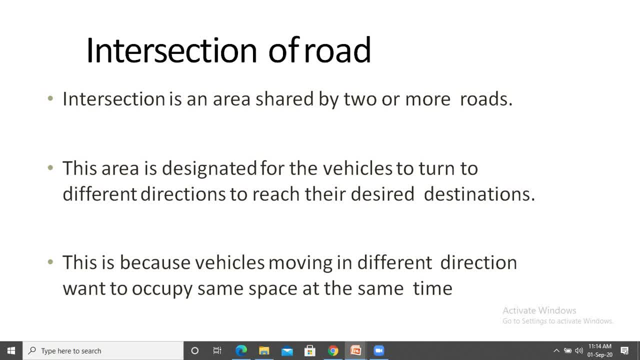 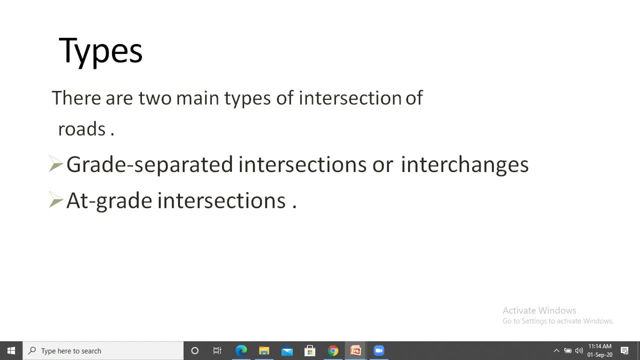 moving in different direction. we wanted to occupy some space at the same time, so we need to provide the direction of the vehicle. so, guys, so how? two types is there here, main two types of intersection of roads? is there so a grade separate intersection or interchanges, you can say in second one, at a grade intersections? 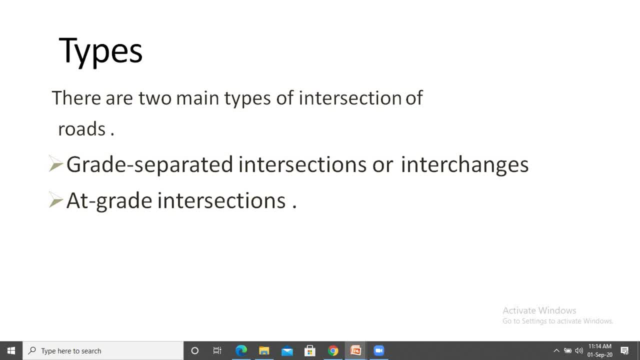 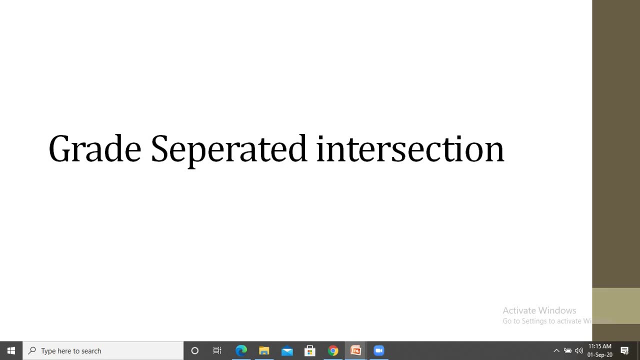 so how to types is there here. so we will discuss a little bit information regarding this grade separate and as well as the at a grade intersection. so, guys, this is a grade separate intersection. the intersecting roads are separated by C and we will discuss this in another lecture also, so we can take a look at class if at. 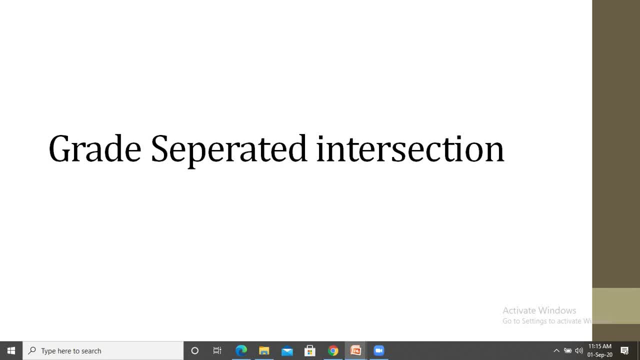 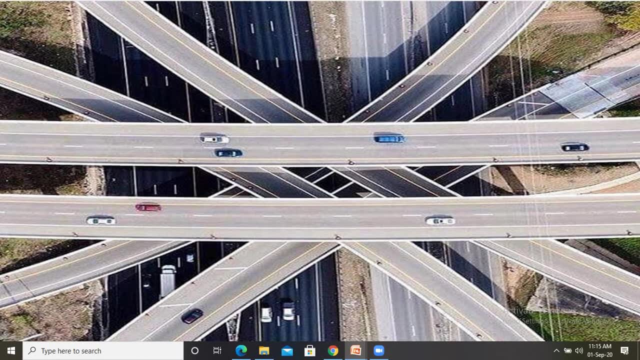 we do see that noise, Royal noise, but, as I already said that this is a grade separate intersection, so it's right we are going to talk about that also. so that's it and that means for let's look at different made this year. so it's a grad duplicate intersection and the main thing is how to determine the location. but during last year we were processing the process, then returning vehicles through the system. Yes, guys, this is a picture. so, without disturbing, without any kind of collision, we are moving or we are providing our transportation system, medical here, different stages, we are constructing, so according to that, we can move any 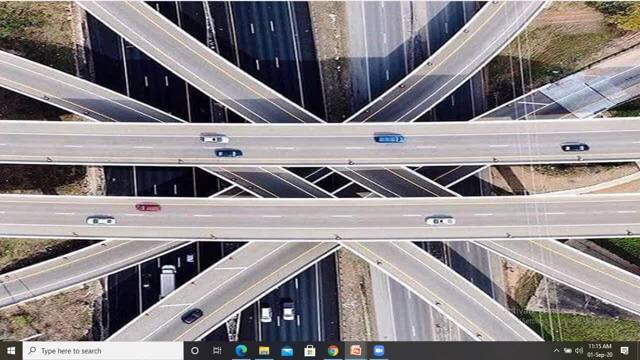 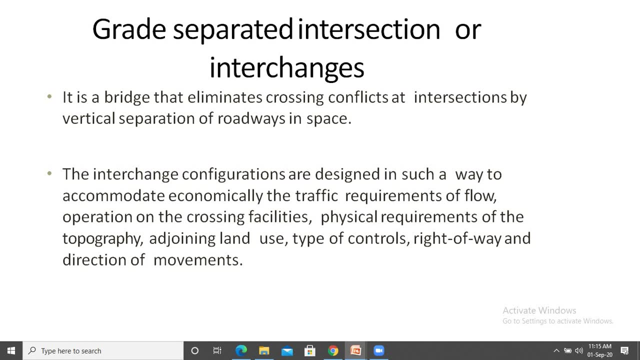 any kind of delay time. so we are moving with the safely, without the traffic flow or any kind of the delay over there. so it is a bridge that eliminates crossing conflicts at intersection by vehicle separation of road waste in space and the interchange configurations are designed in such a 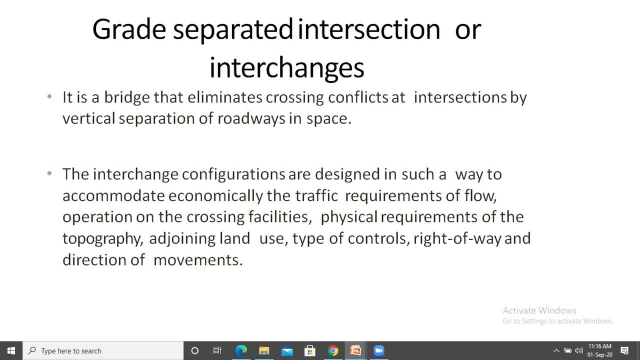 way to accommodate economically the traffic requirements of flow operation on the crossing facilities, physical requirements of the topography, attrying the land use, type of controls, right of way and direction of movement. so these all kind of the parameters we need to take into account and we need to build in a proper channel. then only it is. 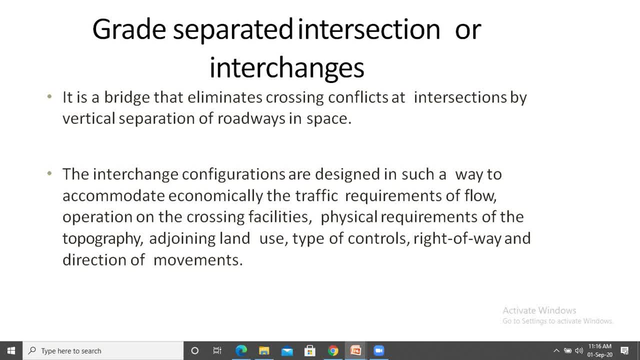 fulfill the road users, whatever may be, if you are not providing any good manner, so going to face lot of the problem, especially geometrical designs. so speeds and speed limits are not good. we need to do required alignments as well as the sight distances. so that is. 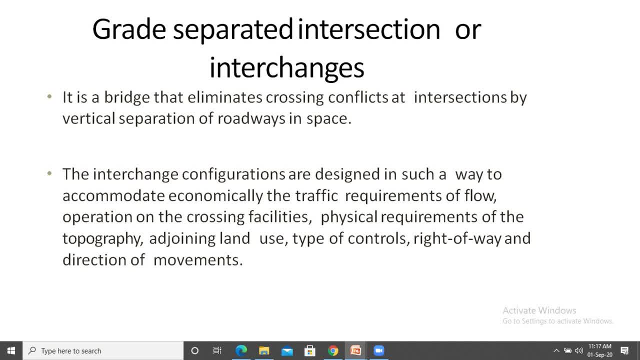 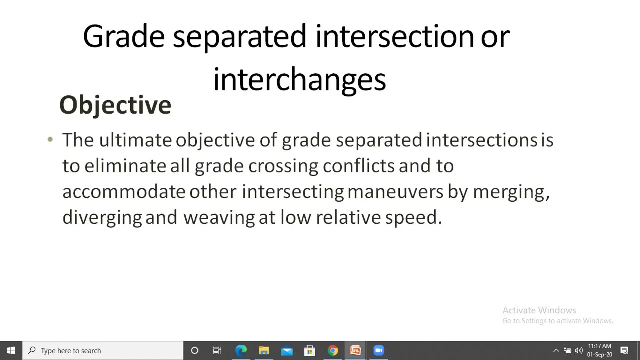 stopping sight distance, overtaking sight distance, intermediate sight distance. so these all kind of the parameters we need to take: accident studies, speed study, delay study, origin and destination study, these all kind of the information we need to study. then only we need to build up these grade separated sections. so main: 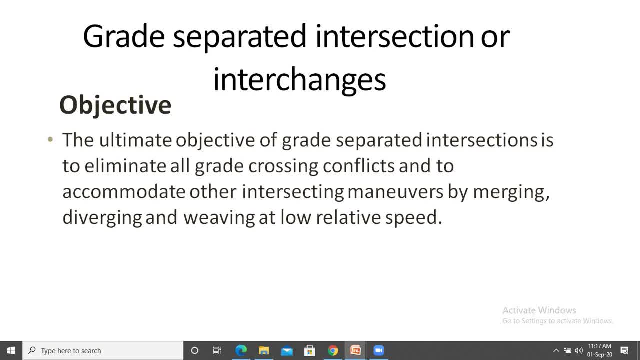 objective is. the ultimate objective of grade separated intersections is to eliminate all grade crossing conflict and to accommodate other intersecting maneuvers by merging, diverging and weaving at a low relative speed. guys, already we are discussing in previous unit merging, diverging and weaving, all those things we are discussed in previous class, so how it is happened. so some of 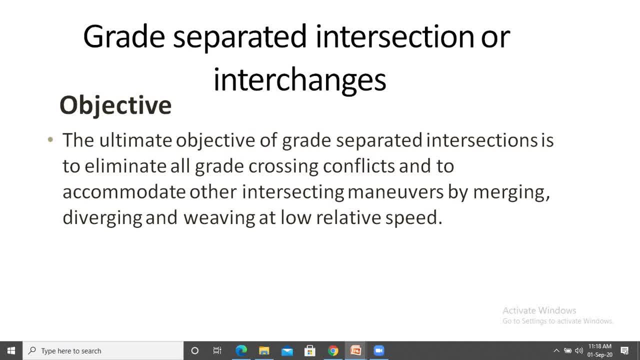 the roads are came from formal village to the joining to expressway or highway or national highway. so that is the emerging, so diverging. is there something is moving some National Highway to some village road and weaving services will take place, these countries, so whatever it may be. so these kind of 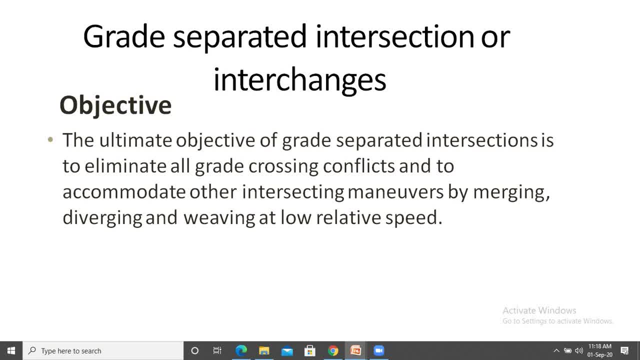 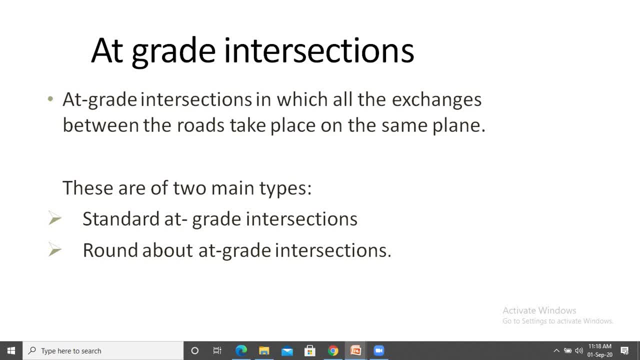 parameters is going on at a low relative speed in grade separated intersection. okay guys. next one is the at a grade intersections. that's a retrograde intersection in which all the exchanges between the roads takes place on the same plane. so we can say here, these includes all roads. 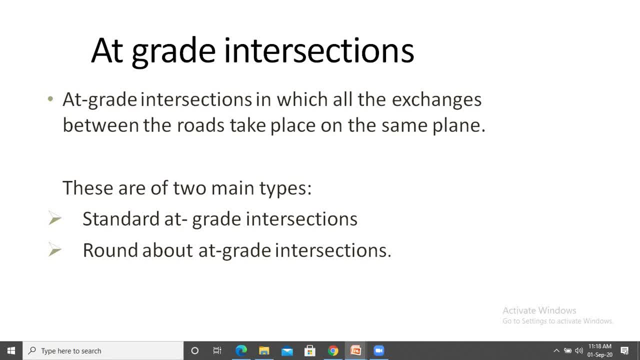 which meet at a more or less the same level. the traffic maneuvers like merging, diverging and crossing are involved in the intersections at so merging, diverging, as well as weaving these three parameters, meeting at a particular point, so that point is known as the at a grade intersection. so our indian roads obviously, so maximum not. 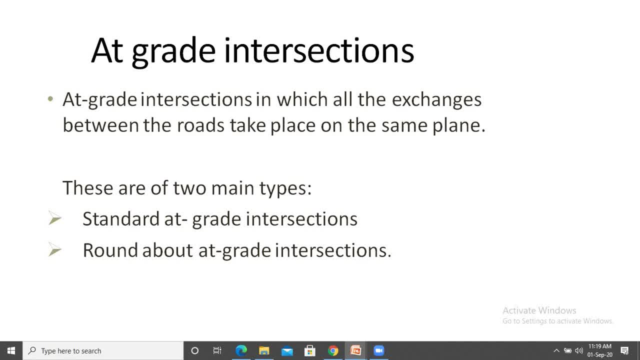 indian road in world maximum. in india we are using 90 percent integrated only, but in other countries a little bit uh. so where it is required they are building at a grade intersection in less percentage. so maximum they are using grade separate intersection. so means without any delay. 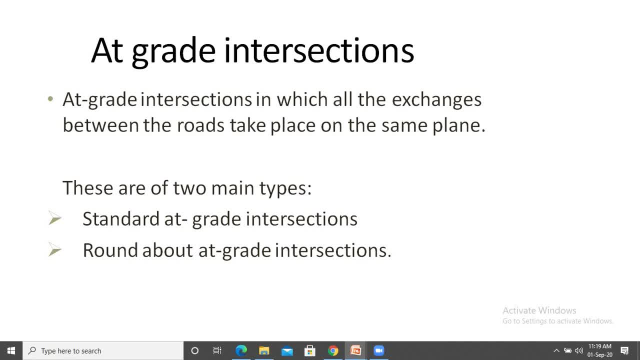 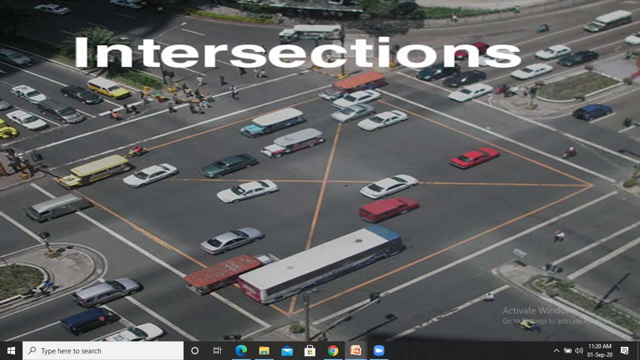 whatever it may be, or without any effect of graphic flow, they overcome the problem and they are moving with the safe. so that is the integrate intersection. so there are two main types, is there, guys, here in at grade intersection? one is a standard integrated section and round about integrated intersection. how two types is that? so, guys, this is the uh at a grade intersection. 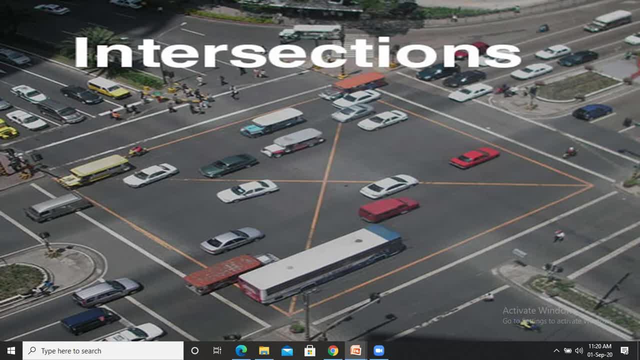 is there. so four roads meeting at a particular point, so obviously two, or more generally we can say two or more so. so lot of delay is going on like this. so with the at a grade intersection, so four lane road is there. now, for example, we are allowing only one side of the vehicles. 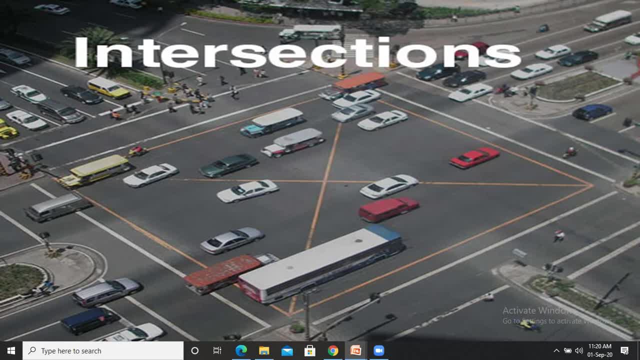 flight, so remaining three sides of the people they stop at particular time, i wonder some to one, to two minutes. so this type of problem is going to happen. so that's why we need to take, uh, great, separate intersection. that is a better. so delay is maximum here. this is the picture. this is the intersections integrated. 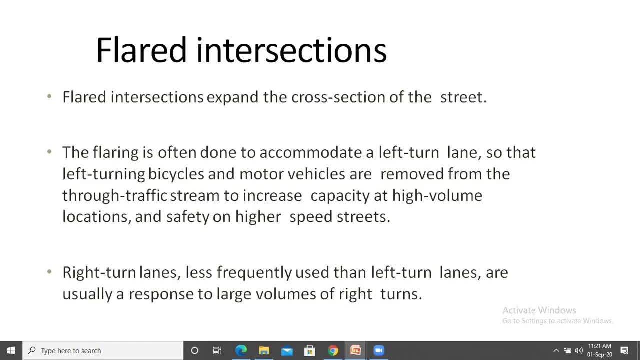 so flared intersection is there, expand to cross section of the street. in this case the flaring is often done to accommodate left, so the left turning bicycles and motor vehicles are removed from the through traffic streams to increase capacity at a high volume location and safety on player speed street. yeah, we. 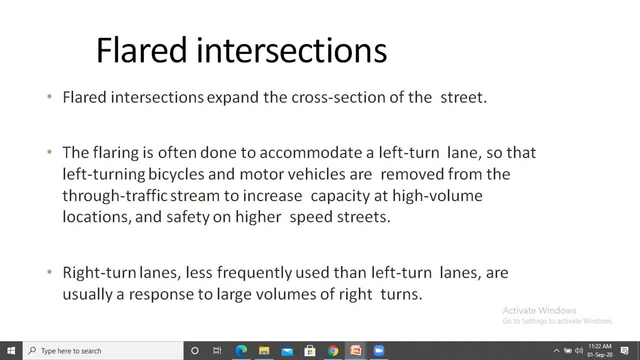 can take this particular point so separate the bicycles and motor vehicles in a particular lane moved from the traffic stream. then we can reduce a little bit traffic flow on that particular place and that is a left turn lane. so if i take a right turn lane so less frequency used that left turn lanes are usually a response to. 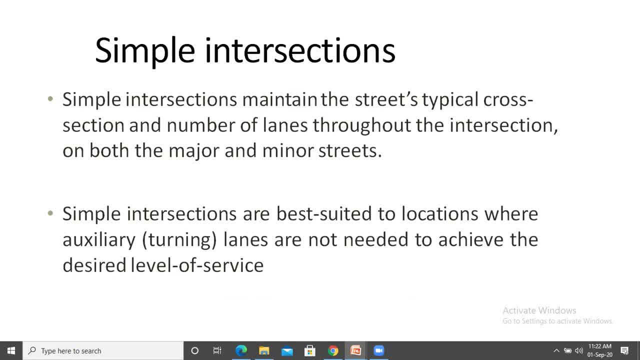 traffic. it is a good idea to have a large volume of light, which is the one point, and simple intersection is there. simple intersection is maintained. the street, typical cross section and number of lanes through the intersection on both the major and minor streets, and simple intersection are set up and 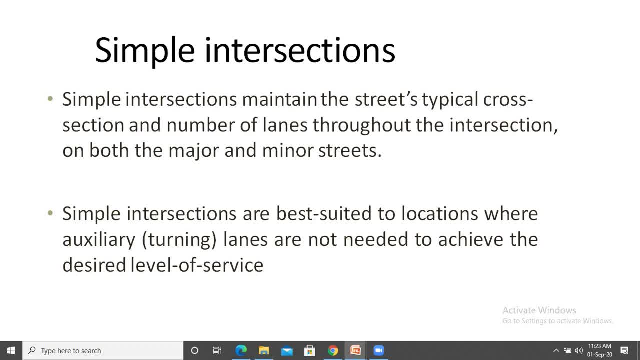 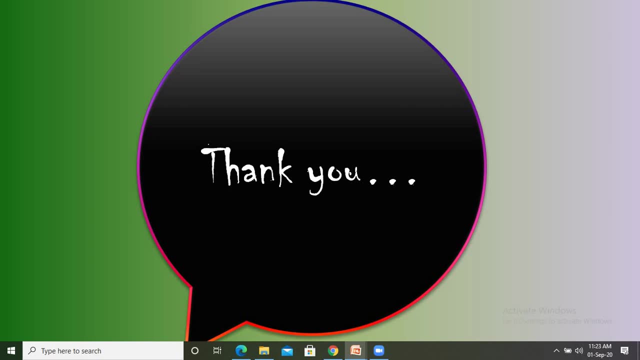 where auxiliary lanes are not needed to achieve the desired level of services. so this is the information, guys, regarding the intersections at the grade intersection, as well as the grade separate intersection. so this is the information and how. how more information is there about it? grade and grade separation section. we will briefly discuss this individual topic from next. class. thank you.